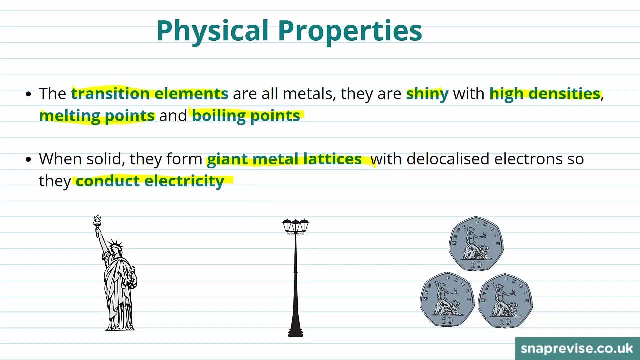 So these are all typical properties of the transition metal. Because of things like their high densities and their shininess, they're used a lot in electronics. They're also used in objects you'll see around. For example, the Statue of Liberty contains lots of copper. 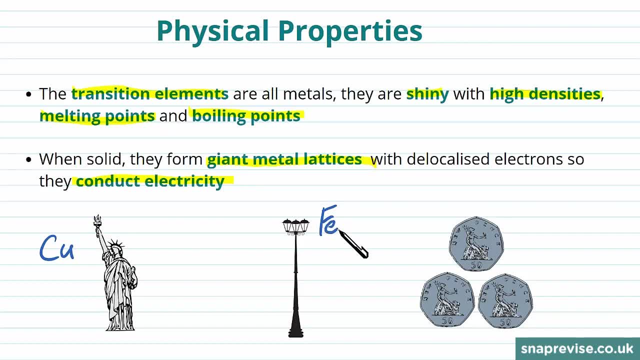 lampposts tend to contain lots of iron and 50 pence pieces contain nickel, All of which are transition elements and all of which have the properties that make these items useful to us. You wouldn't want bendy 50 pence pieces. 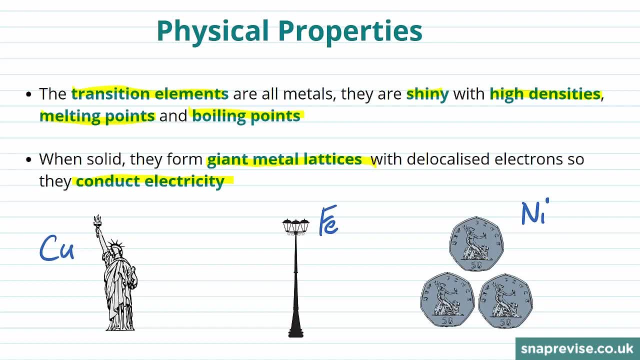 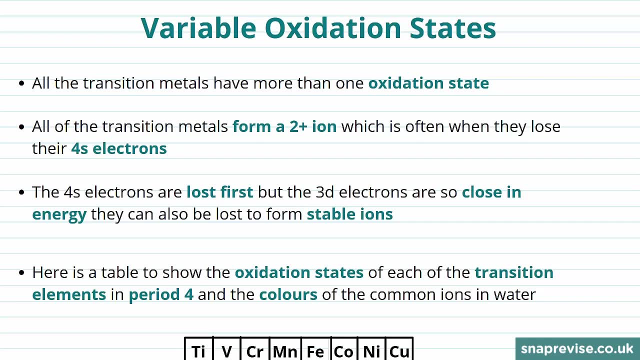 or a statue of the Lady of Liberty that's likely to melt on a hot day. One of the first key chemical properties of transition metals we're going to look at is the fact that all transition metals have more than one oxidation state. In fact, having many oxidation states is a property that's characteristic of transition metals. 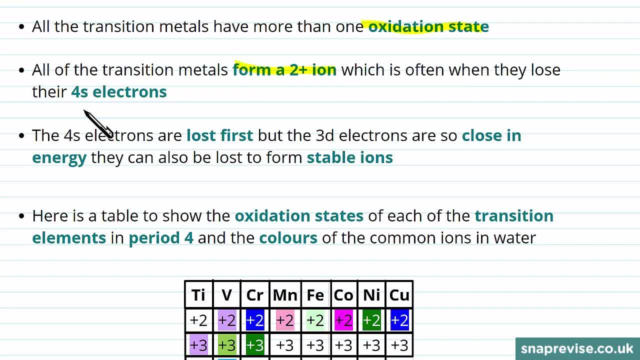 All of them form a 2 plus ion, which is often when they lose their 4s electrons. Remember there are two electrons in the 4s orbital, so losing those will form a 2 plus ion. The 4s electrons are lost first. remember. 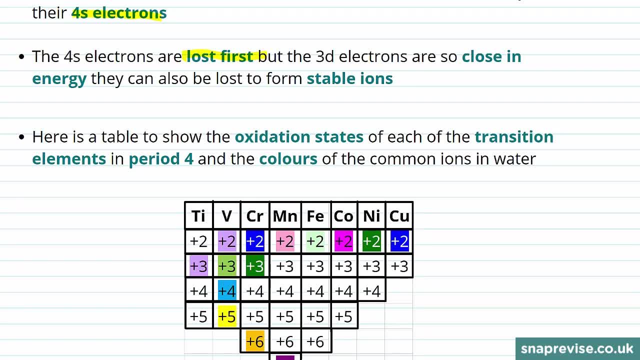 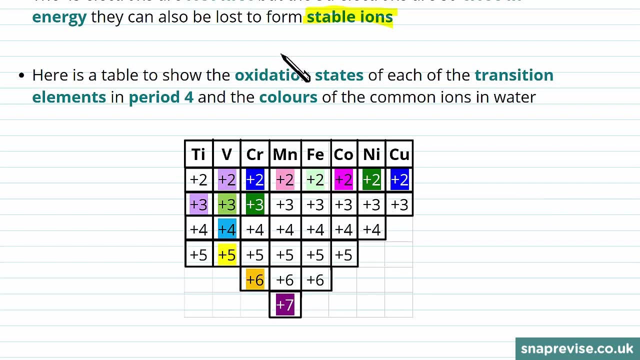 but because the energy levels of the 3d electrons are so close, the 3d electrons can also be lost to form stable ions for the transition metals. Remember that's what makes them transition metals: the fact that they can lose some of their 3d electrons and form stable ions. 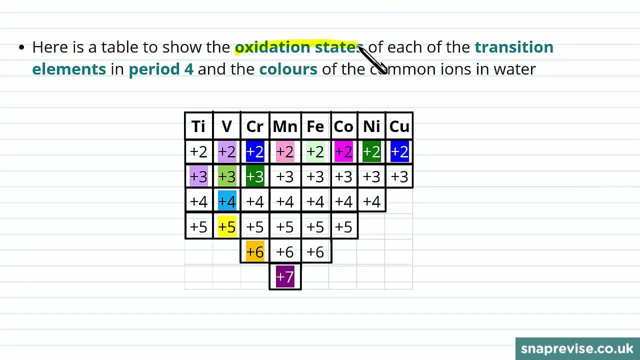 So here's a table that summarises the odds of a transition metal being lost. Here are the oxidation states of all of the transition elements that are located in period 4 of the periodic table. This is the first row of transition elements in the periodic table. 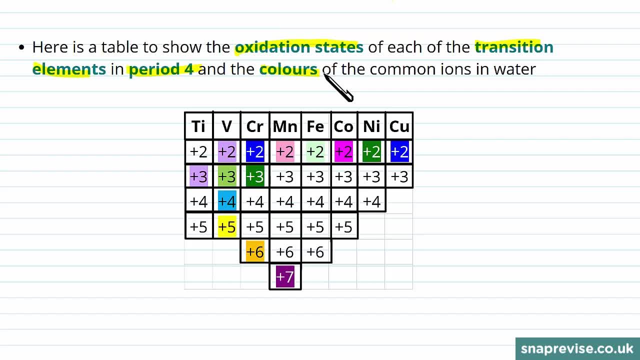 The colours of some of the common ions that you'll come across in water are also shown. You should already be familiar with some of these colours. For example, manganese 7 plus, which is in potassium permanganate, has a purple colour. 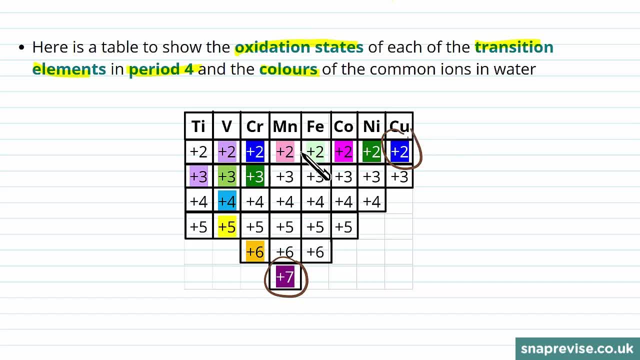 Copper 2 plus in solution has a blue colour, Iron 2 plus has a pale green colour And chromium 6 plus, which is in dichromate, has an orange colour. The rest of them you will come across and meet at some point in the course. 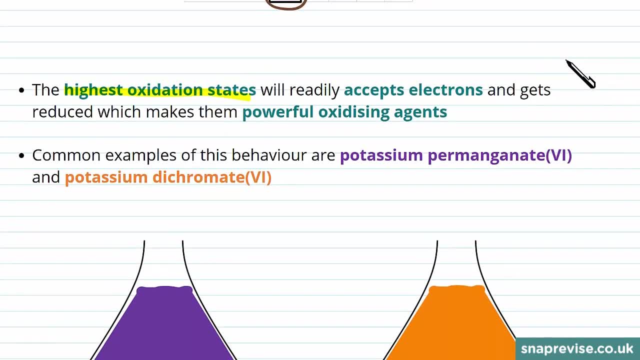 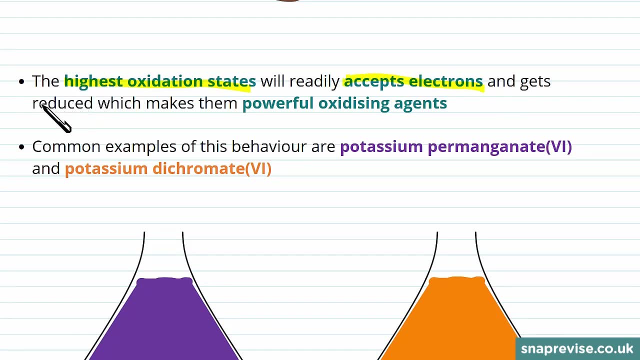 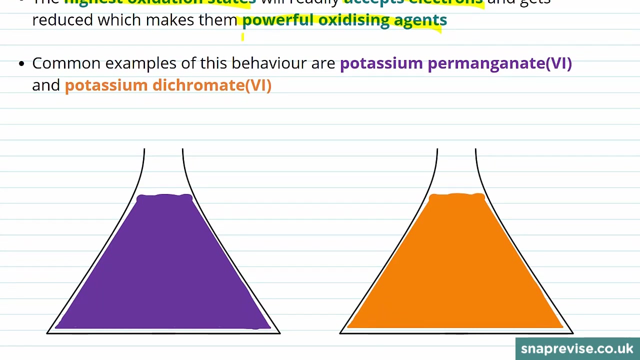 The highest oxidation states of the transition metals will readily accept electrons to lower their oxidation states and this means they are reduced because they are easily reduced. This makes them powerful oxidising agents because they will take those electrons from elsewhere. You should have already encountered the oxidising agents potassium permanganate and potassium dichromate. 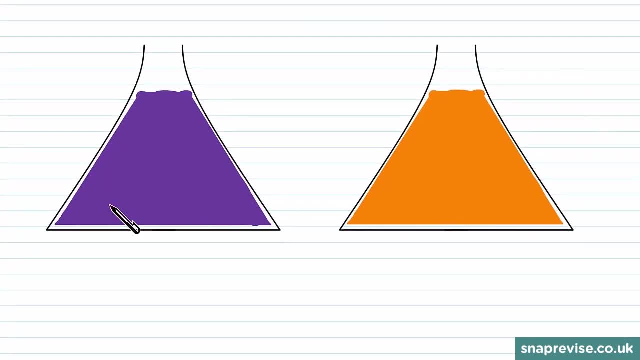 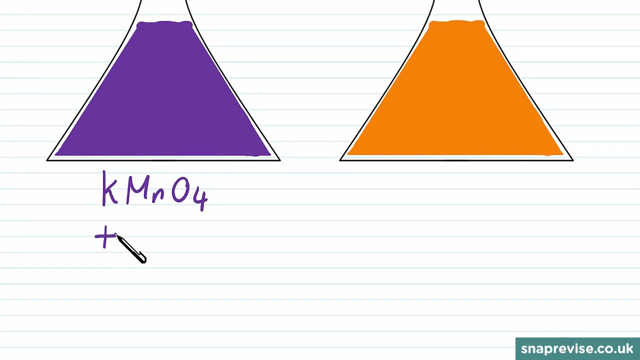 We cover these in our video on redox titrations. Potassium permanganate has the formula KMnO4, and this is a purple solution. We can see the oxidation number of the manganese here by realising that potassium carries a 1 plus charge. 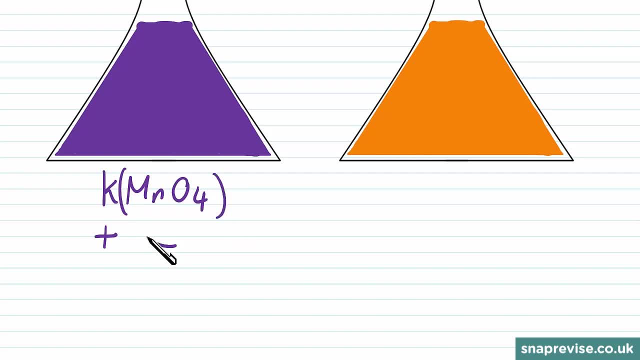 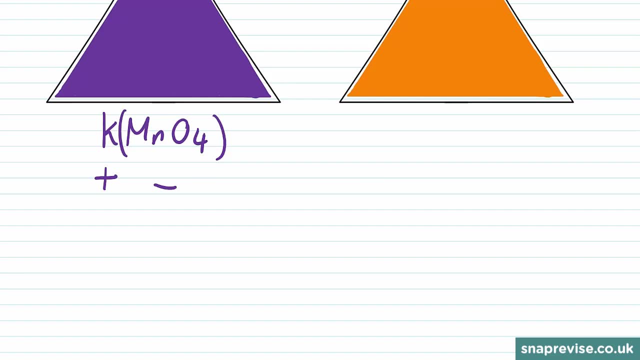 so the manganese ion shown here must have a 1 minus charge. Oxygen has an oxidation number of 2 minus per oxygen, so we have 4 lots of 2 minus for the oxygens, which gives us 8 minus. The manganese must counteract some of this 8 minus. 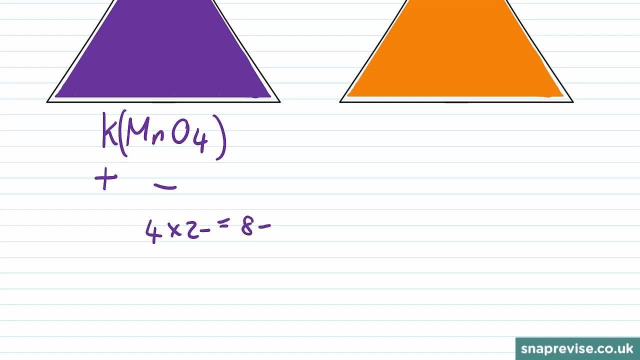 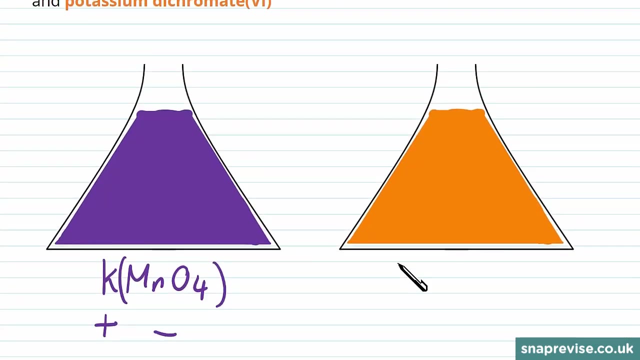 to give an overall charge and so oxidation number of the manganate ion of 1 minus. so the manganese must be 7 plus, which we saw earlier in our table. Similarly for potassium dichromate, which has the formula K2Cr2O7,. 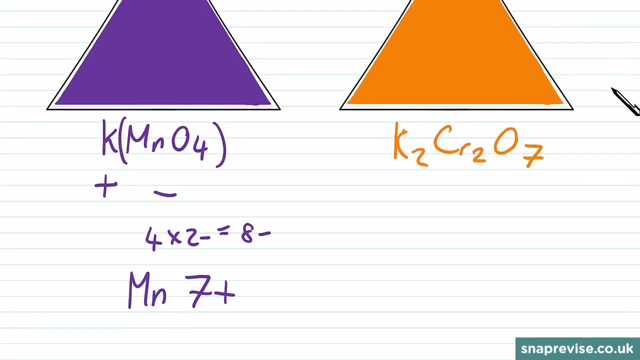 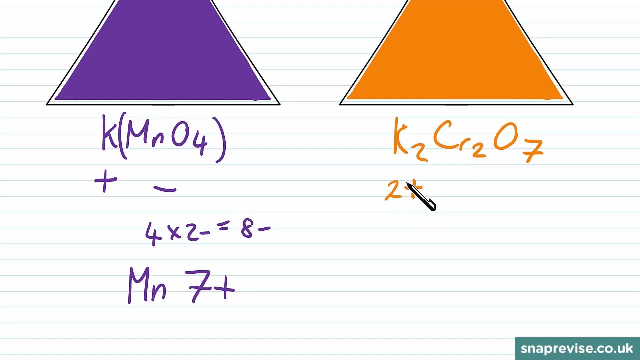 we can use logic to work out the oxidation number of the chromium ion. here So the potassium, because there's 2 of them, will provide a 2 plus charge. here, so the dichromate ion, Cr2O7, must provide a charge of 2 minus. 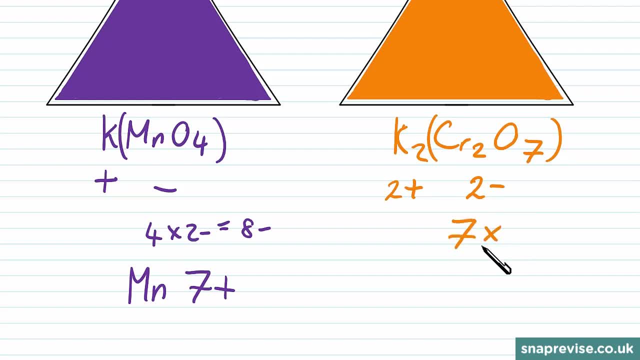 If we then consider the oxygens again, we have 7 lots of 2 minus, which gives us 14 minus. so we need the oxidation of the chromium ions. to take this 14 minus to 2 minus 12 plus would do this if we had 12 plus from the chromiums. 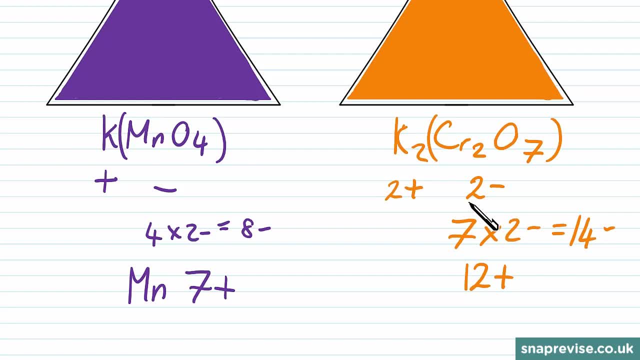 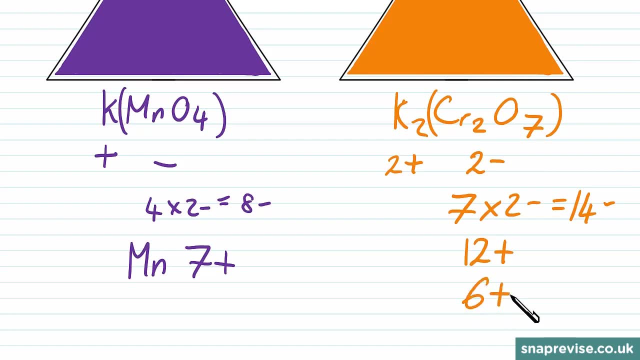 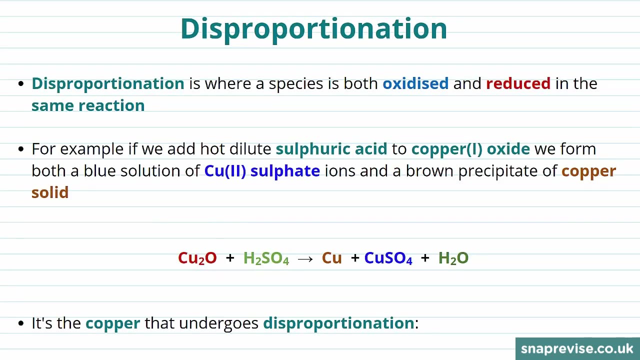 and 14 minus from the oxygens, we would have 2 minus. overall. There are 2 chromium ions, however, so this is why each one of them has an oxidation number of 6 plus. Because of their multiple oxidation states, transition metals can undergo disproportionation.